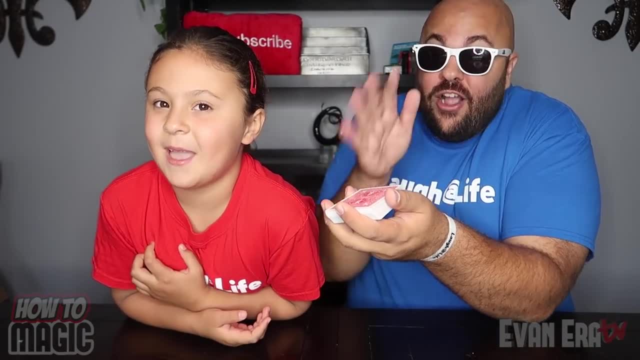 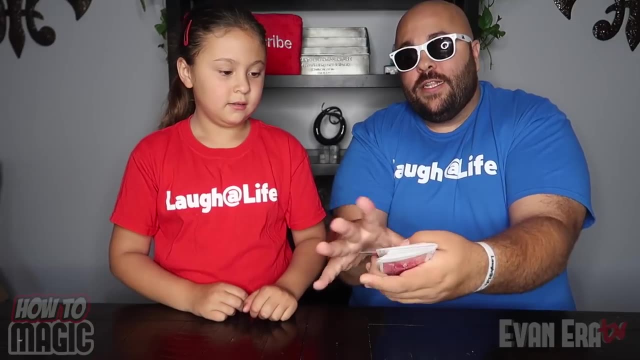 These are magic tricks that I can do, Yes, And everybody else All right. so this first one is a fun card trick. Pick a card, any card, my dear, any one you want. They're all different, right? They're not all the same card. 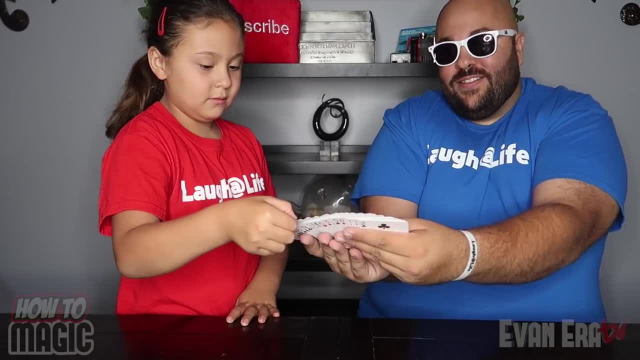 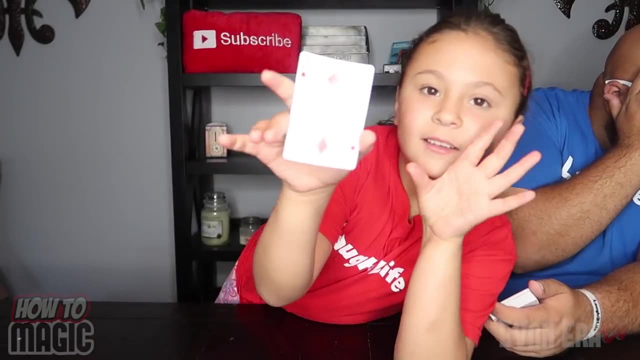 It's not a trick like that. So just pick out any card you want from this deck, just a single one, and take a look, Show the camera so that they can see. Do not see that I will not look, I will avert my eyes. 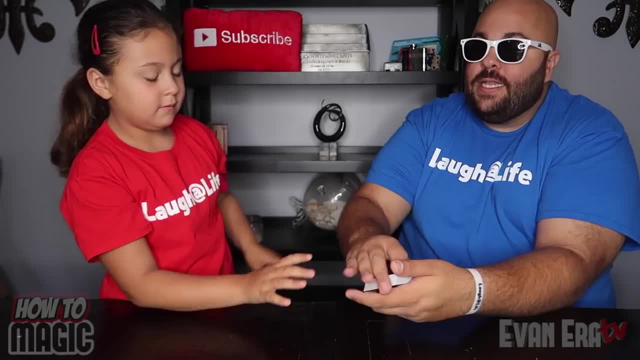 Just get a good look at it. Put it right there on top of the deck. Perfect, Now you have the card in your mind, correct? I'm going to cut it into the middle of the pack, just like this. Now I want to ask you a question. 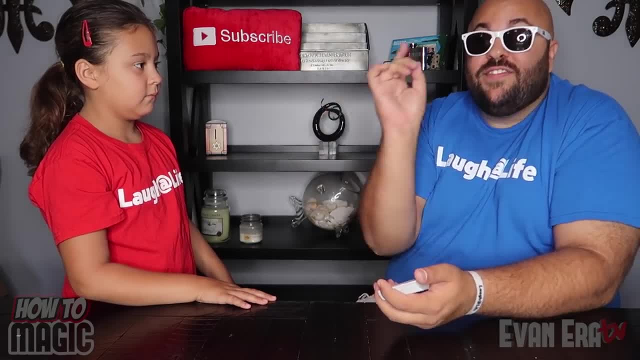 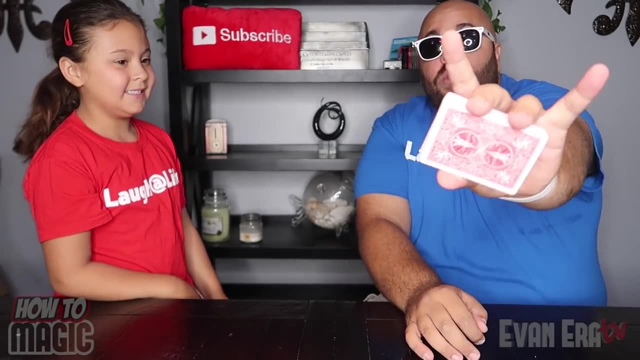 Do you know how many cards are in a deck? 30. Close, It's actually- 15!. No, 52. Five, 52 is the correct answer. So you only picked one card out of the deck, though, right. 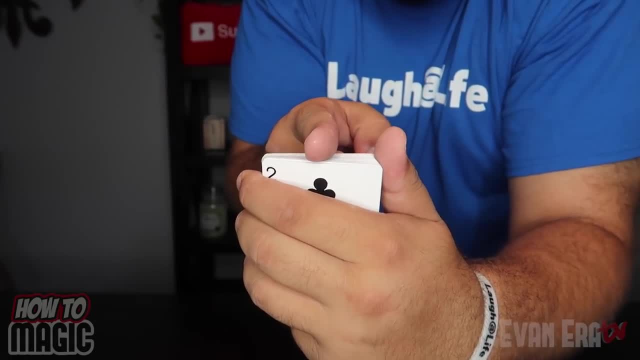 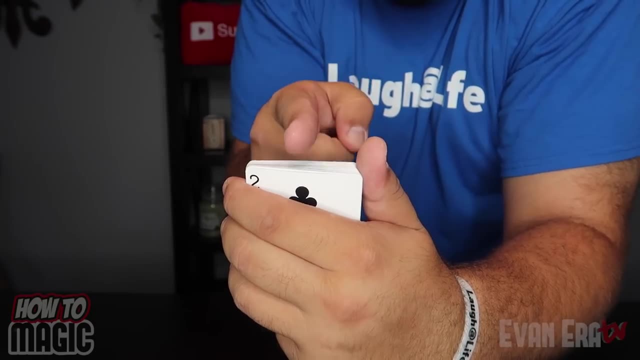 See, You can see this happen. If I put my finger on top of the deck just like this, look, I can get it to kind of like a stick and it looks like one card is just rising right out of the deck. Is that your card? 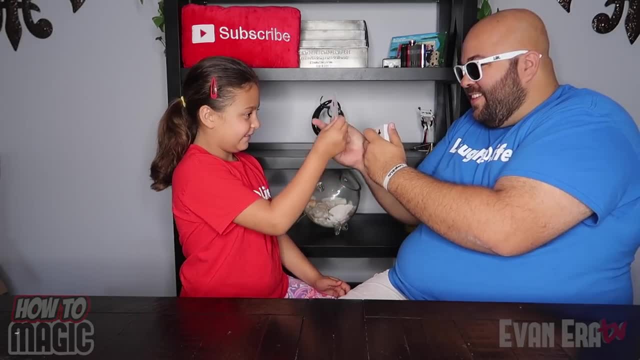 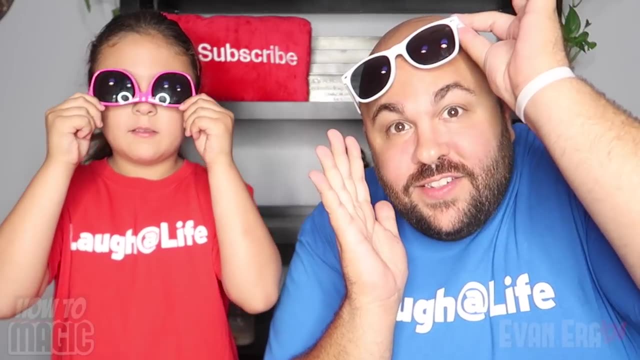 The two of diamonds. Is that good? Is that it? Yeah, All right, Here's how it's done. I'm about to reveal the secret. The secret to this trick is extremely simple, and I'll teach you how it's done right now. 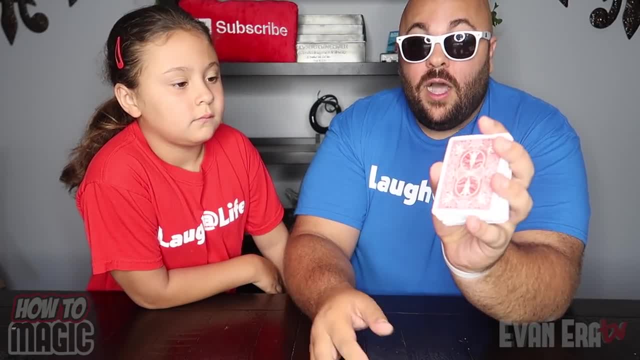 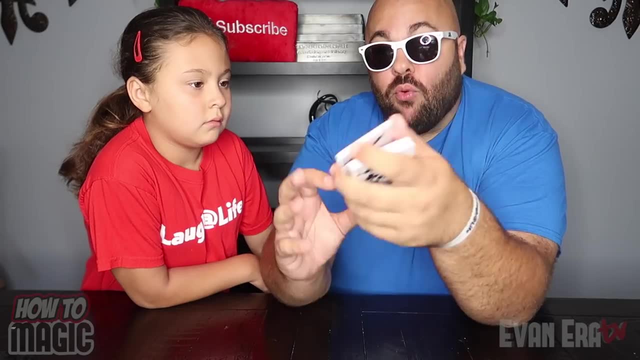 So you take the card, it goes on top of the deck- okay, So it goes on top and you tell them that you're going to cut it. but what you do is you cut the deck and then you leave the cut open. You cut it like this and you hold a break. 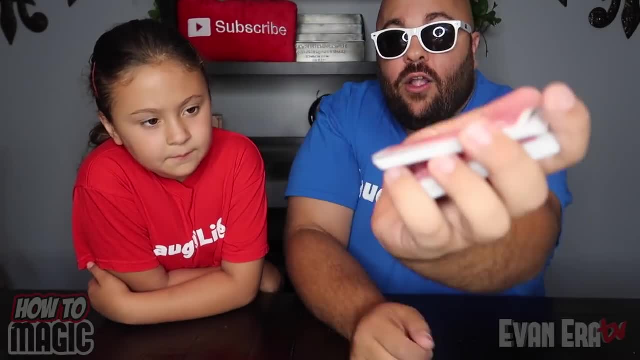 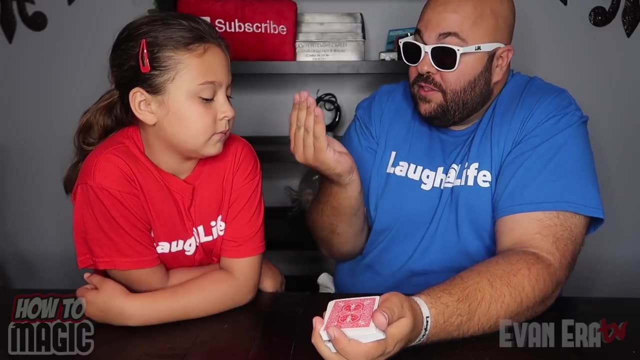 In this case it's the two of diamonds. We're going to leave that two right there with our break, like that, and then we're going to distract them by asking them a question: How many cards are in a deck? And when you ask a question like that, people tend to look you in the eyes to engage with. 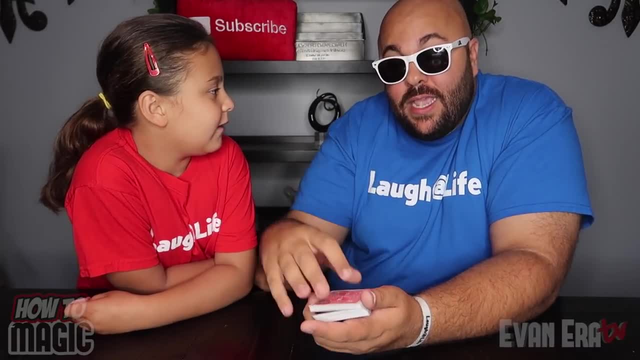 you. So, Ava, how many cards are in the deck? 52.. 52. And when she looks at me, I'm going to cut the cards back so that her card is back on top. You do have to do it quietly. 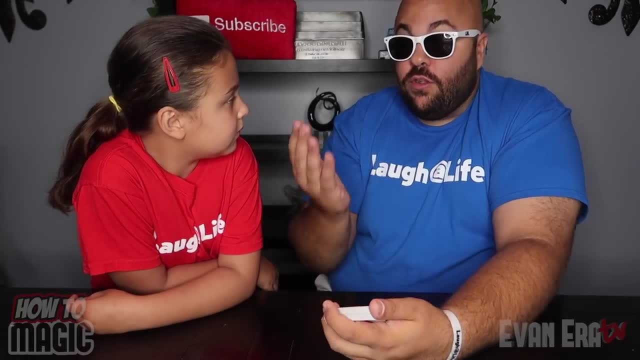 You don't want them to hear you cutting the cards. So you've got it cut. How many cards are in a deck? Okay? So you've got the deck up here. You're just going to quietly cut those back. So now you have their two on top. 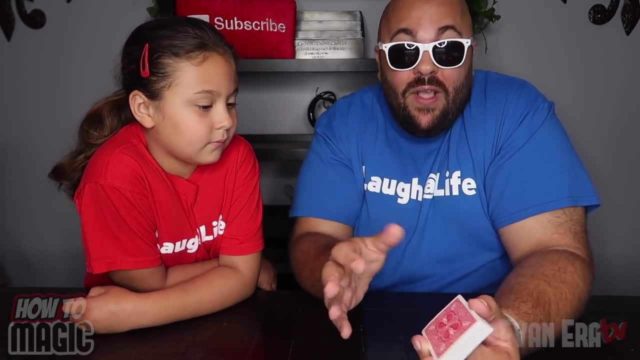 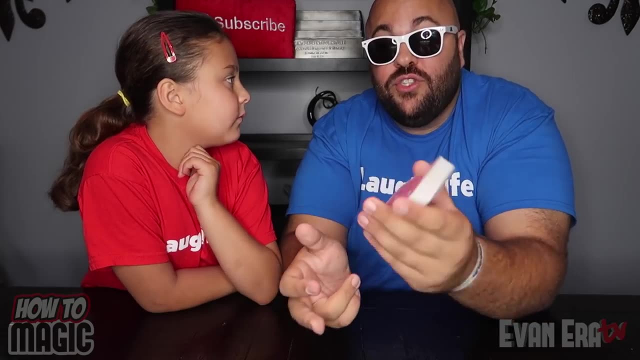 Now here's the really cool part: You don't need any kind of invisible thread or any magnets or any kind of special gimmick deck. You can do this with any deck of cards, anytime, anywhere. It's totally impromptu. So you can take a deck of cards, have them pick one. 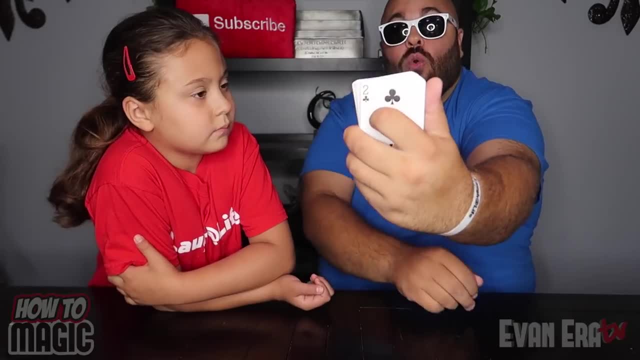 Let's just say, in this case they picked the two of diamonds. You've got to control back to the top of the deck. You're going to hold it like this to present it to your spectator, That's with the bottom card facing them. 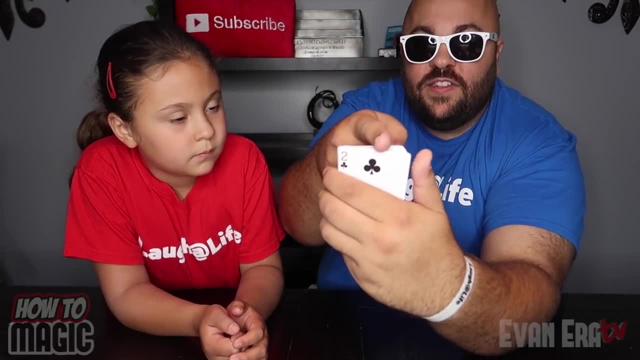 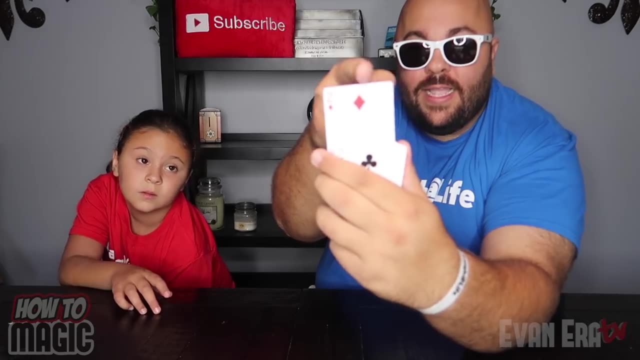 And now you're going to bring your finger to the back like this and you're going to say: watch, we're going to see one card start to do something, Something kind of magical look, and their card just rises up out of the deck like that. 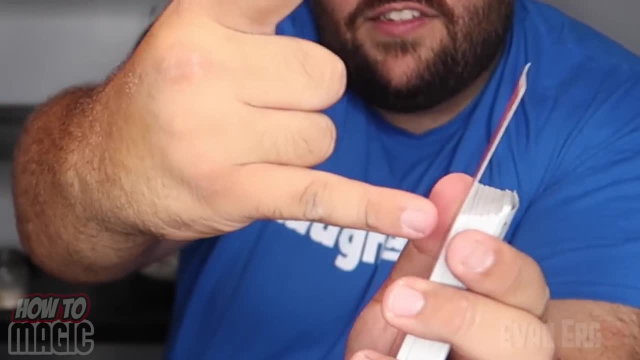 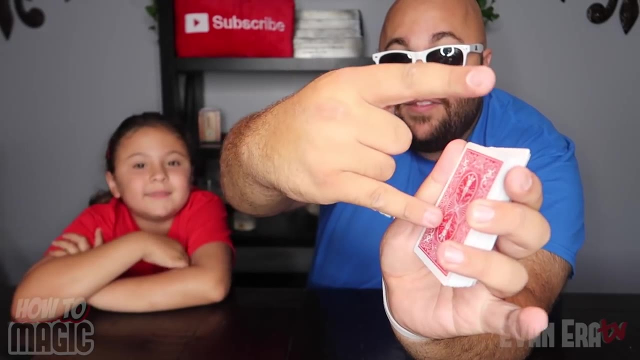 Now, what they don't see is your pinky finger, right here, is contacting the back of that card and pulling it up. So boom, this finger is on top. This finger, the pinky, contacts the back of the card and you just slide it up just like. 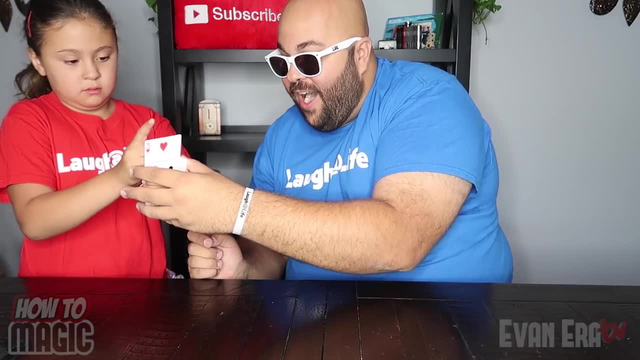 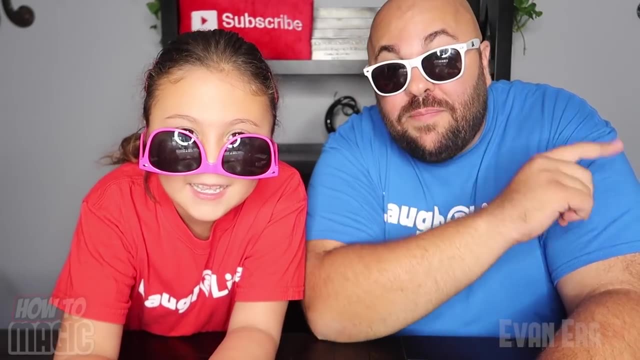 that Isn't that cool. You want to try Push it up. You got it And that is how you do the magic rising card trick. All right, This one is a classic piece of money magic. This is the disappearing coin in the glass of water. 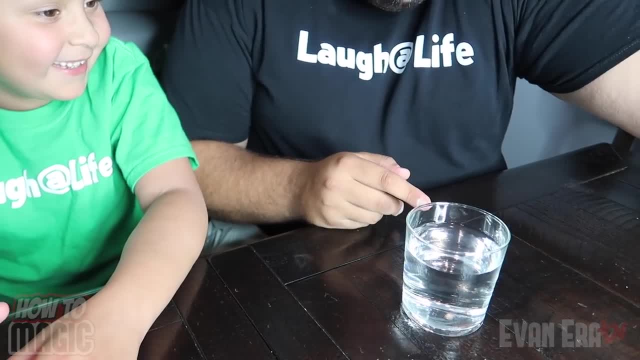 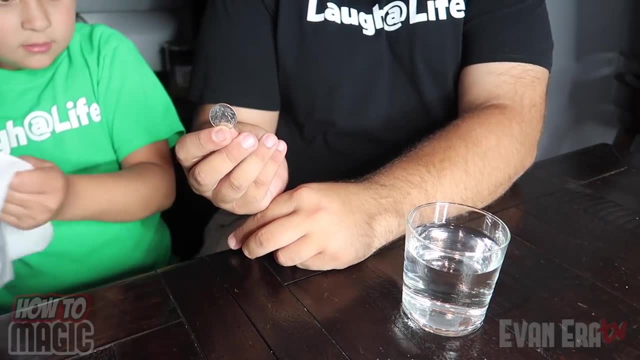 I see the cup of water. Yeah, All right, Check this out. I also have a quarter here and I have a napkin. Inspect the napkin for me. Make sure it's normal. Also inspect the quarter, please. The napkin seem normal. 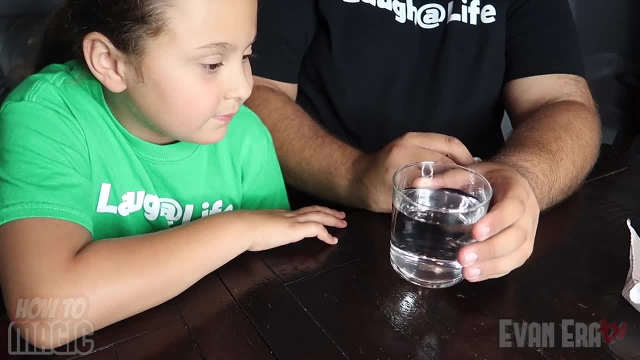 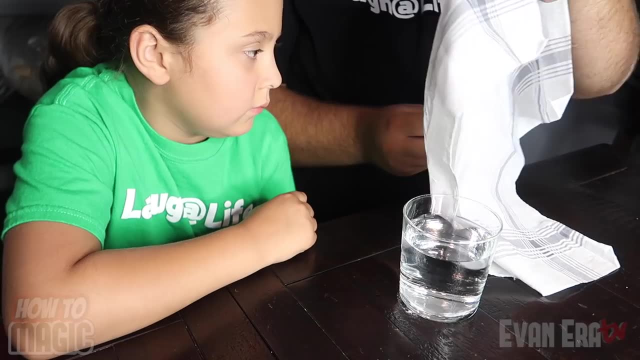 Yep, Okay, Normal. Yes, Glass of water appear normal. So we're going to take the quarter and we're actually going to put it inside this napkin. So I'm going to take the quarter. You can see it going inside the napkin, right? 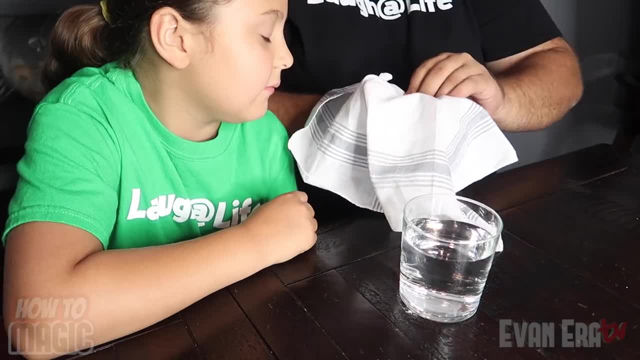 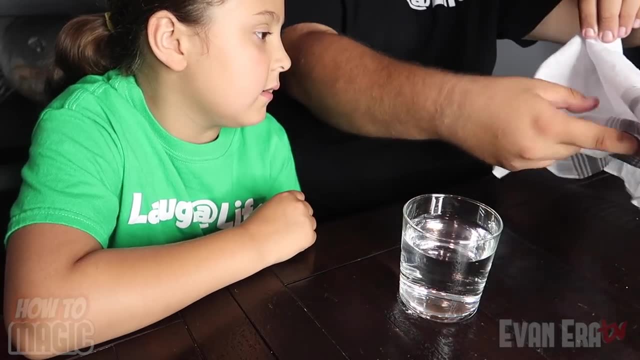 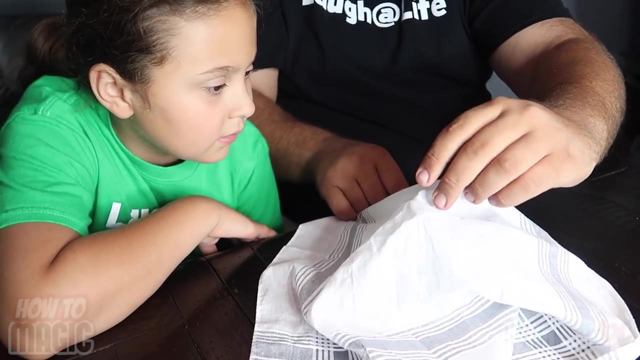 Yes, Okay, So we're going to take it. I'm going to grab the quarter here. See it. I'm going to drape the napkin over the cup. All right, See the quarter. Mm-hmm Watch. 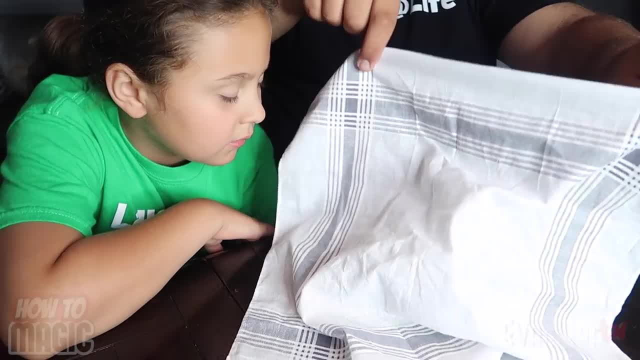 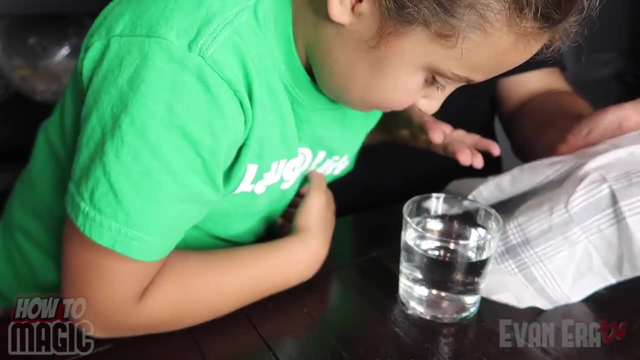 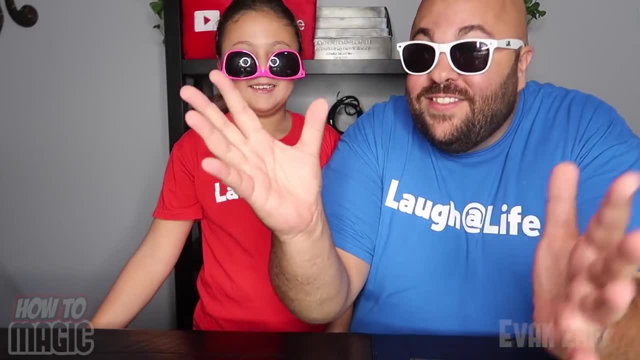 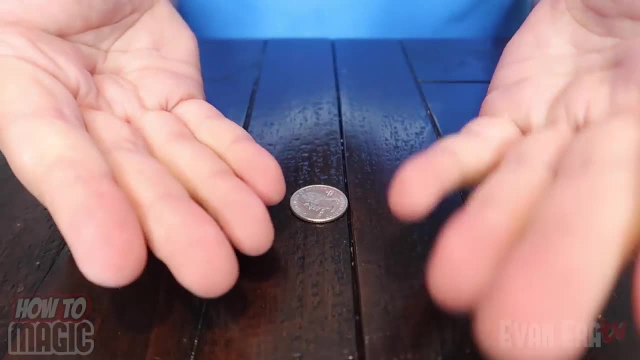 All right, Perfect. That was amazing. All right, guys, Here's the secret behind this amazing magic trick. Okay, Here's what you need for this trick. You need a coin. In this case, I'm using a US quarter, but you can use different currency if you live in. 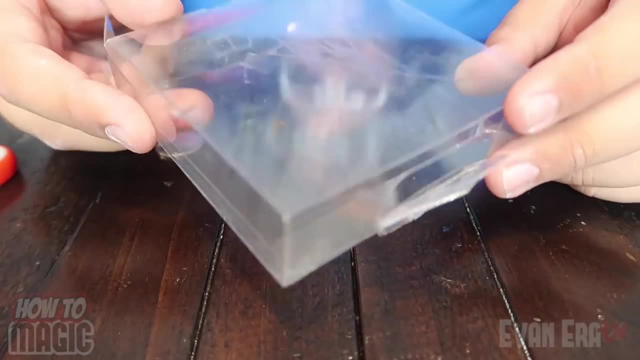 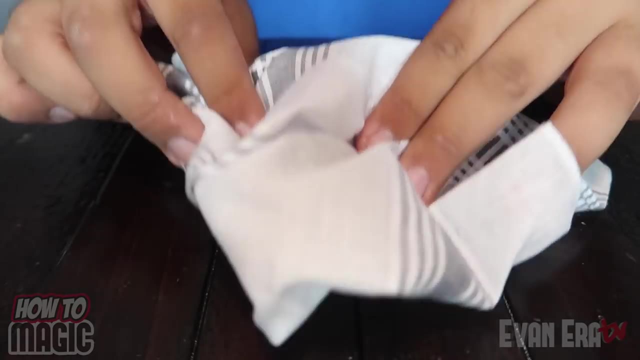 a different country. You'll need some scissors, a piece of clear plastic product packaging. This thicker type of product packaging is what you need. You need this thick plastic, a cup of water and a cloth or paper napkin. Now your first step is to trace around the coin onto the plastic, just like that, so you. 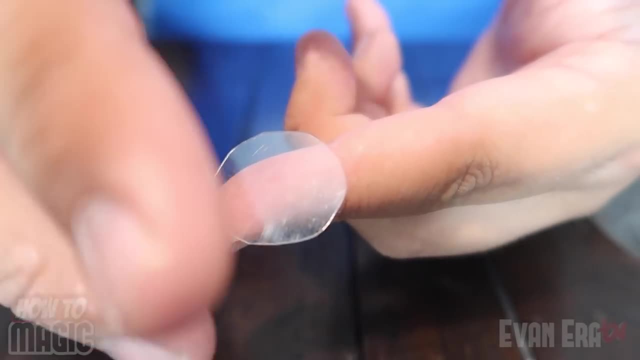 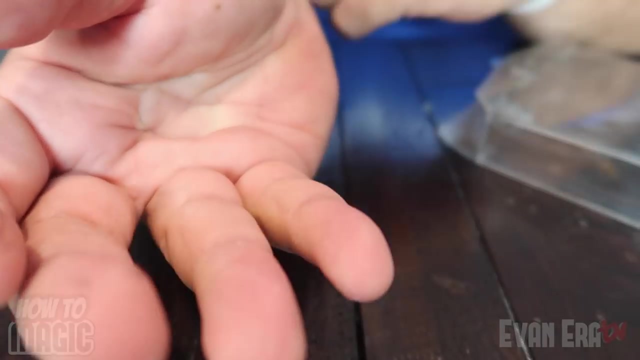 know where to cut. Trim off the excess. Trim off the excess, and now the work is pretty much done. This is what you need to pull off the trick. You're going to conceal this little plastic disc in your hand before the trick starts. 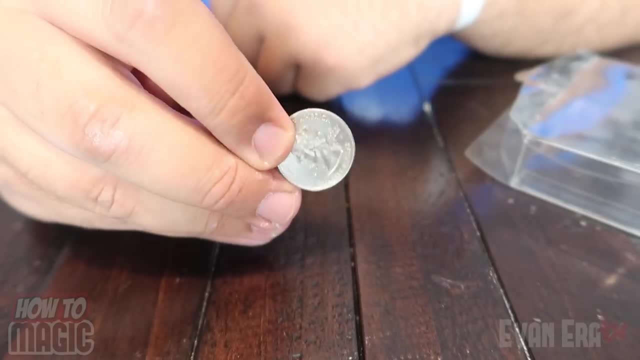 just in a standard palm position like this. Now you're going to hold the coin at your fingertips and present it to the audience, Pull out your glass of water and say: watch, I'm going to take this coin and make it disappear. 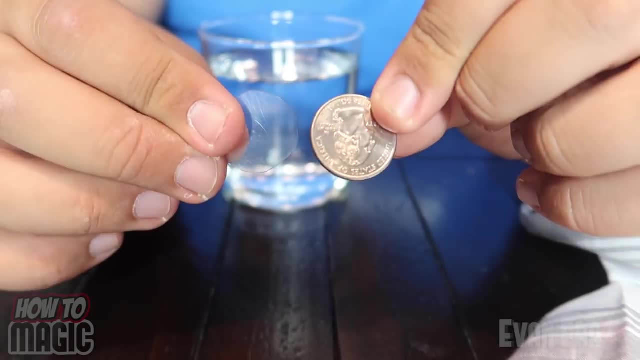 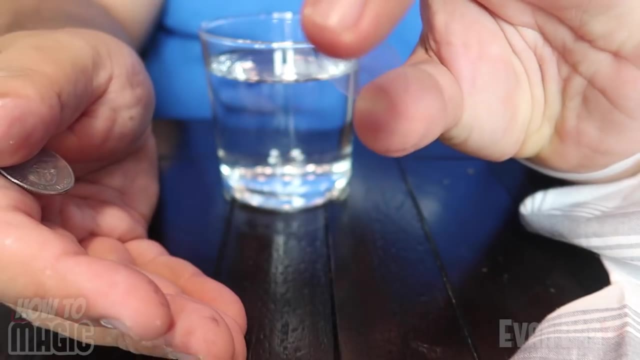 Take your napkin and wrap it around the coin. Now what you're doing under the cover of the napkin is actually switching the coin with the plastic disc. You're going to bring the plastic disc up and grab it with the napkin and leave the 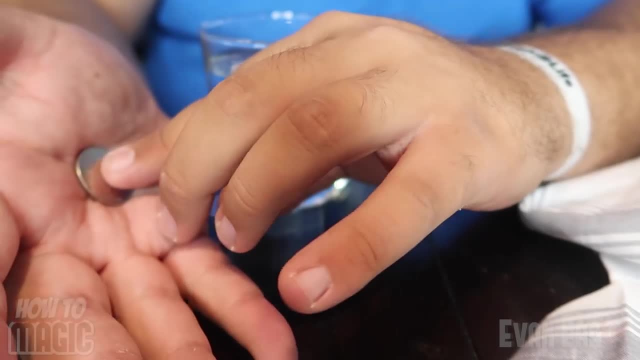 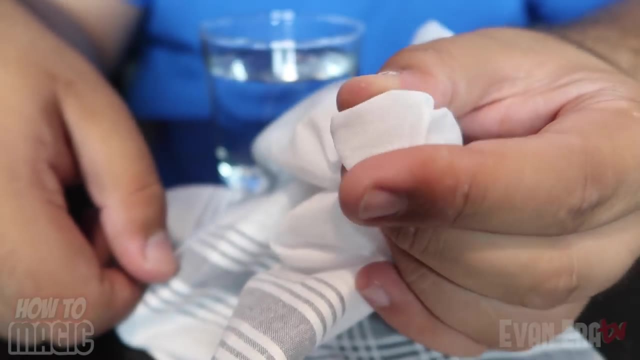 coin in the palm of your hand, switching it to the plastic disc and putting it right back in palm position. Now that you've got the little plastic disc inside of the napkin, it totally looks like the coin, because you cut it to the exact same size. 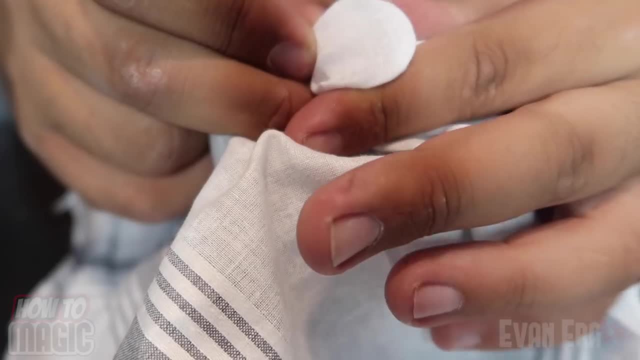 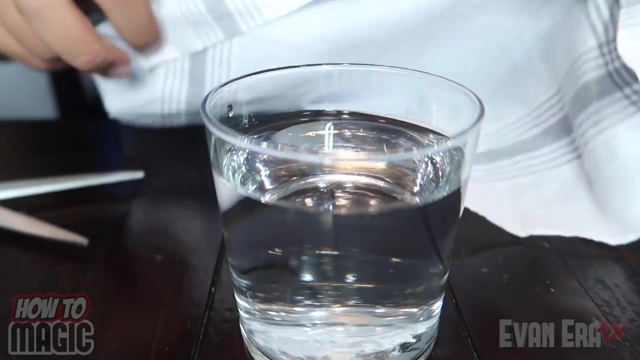 You can show this off to the audience, Say, look, We'll take the coin. Now. they can see the coin inside the napkin. It goes right down inside the cup and you can instantly pull the napkin off and show that the coin has disappeared. 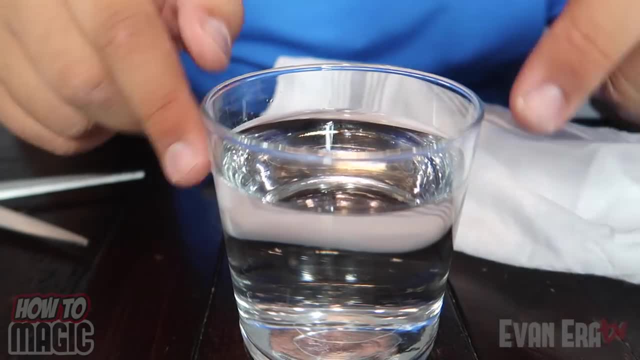 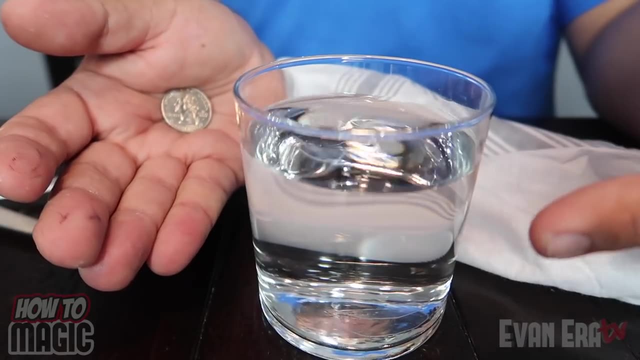 Because the little plastic is clear. it's going to sink to the bottom of the cup and be completely invisible to the spectator. The little piece of plastic just completely disappears into the cup and while their attention is here, you're going to drop this hand to your side and ditch this coin into your pocket. 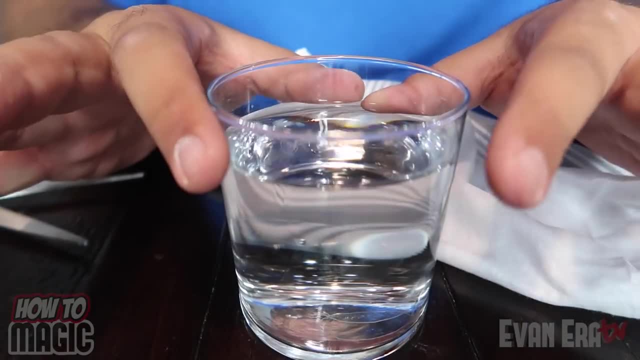 Boom and come right back up to the table to show your hand's empty. Now you're going to do that while everyone's attention is misdirected at the glass. If you look closely, you can barely make out the little piece of plastic in the bottom. 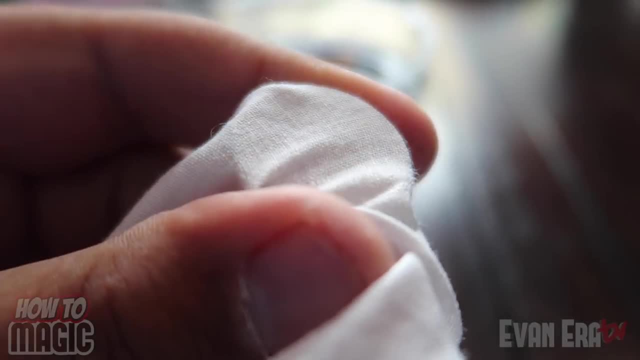 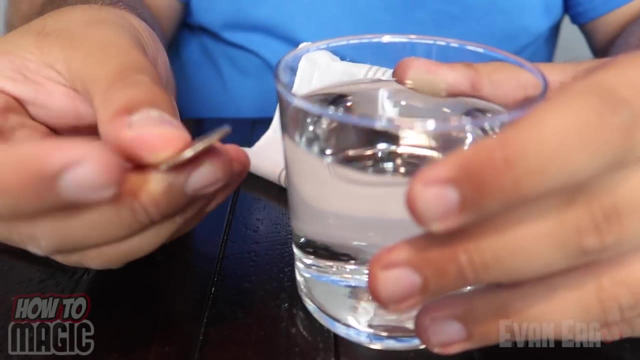 of the cup there Really hard to see. They think they're seeing the coin right there in the napkin. so when it drops into the cup and you immediately pull the napkin off, their mind is going to be absolutely blown. Super easy and fun coin trick that you can do at home right now. 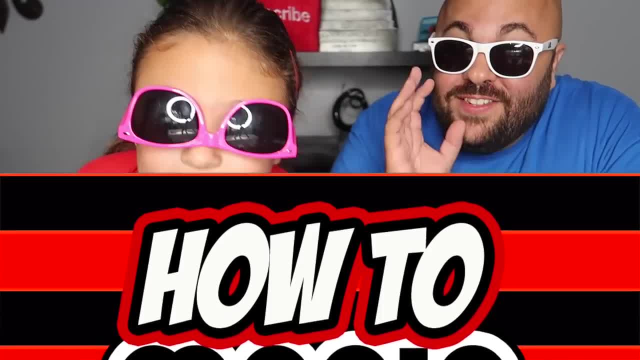 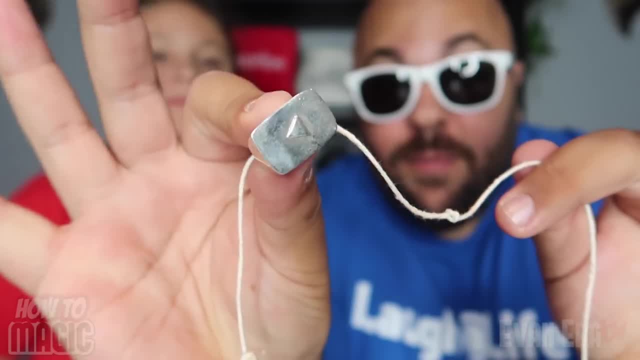 And that is how you do the magic disappearing coin trick. All right, this is a really fun one. You use a ring like someone's finger ring and a piece of string- The ring and string trick. Check it out. Okay, see how I've got my cool YouTube ring right here and I've got it tied on the string. 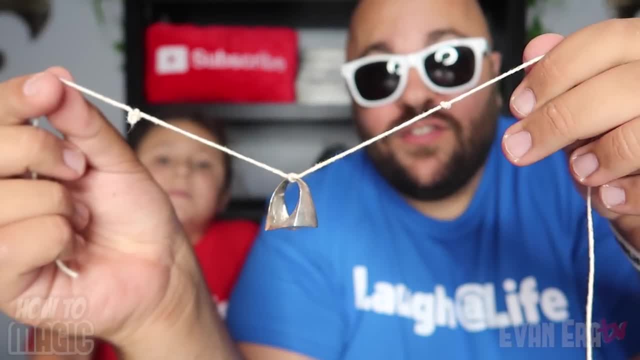 like this: Mm-hmm, All right. so you've got the ring on the string with the three knots and it's tied on the middle one. You see, Mm-hmm, Now watch On the count of three. you're going to see this happen. 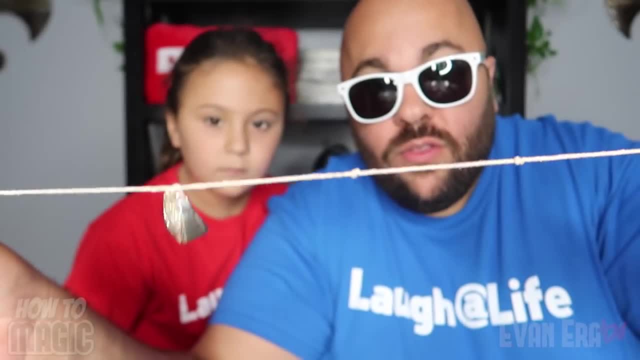 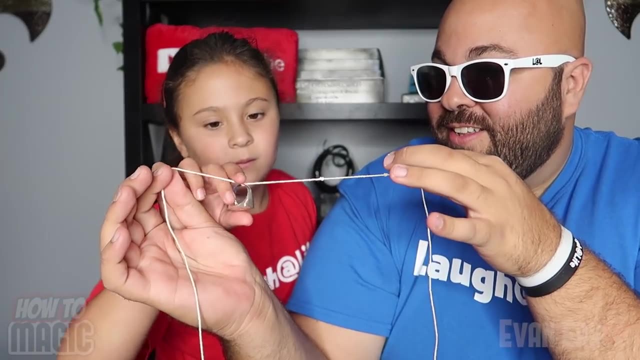 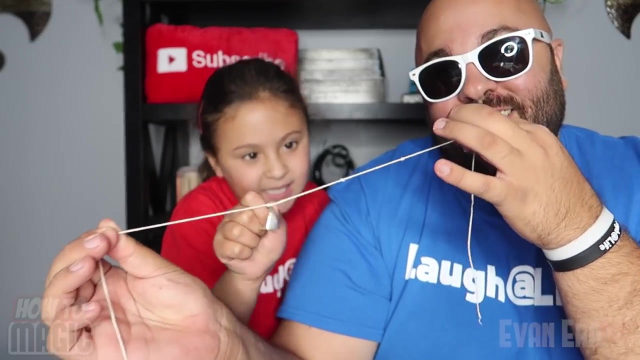 Ready. One, two, three. Boom, One, two, three And it jumps to the other knot. Look you see, Yeah, It's still tied on there. Check it out. Here's the secret behind this easy magic trick. 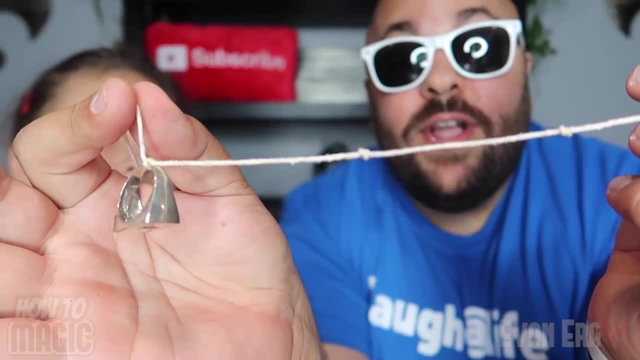 This is a really easy one that you guys can do at home, and, Ava, you can do it too. So you have three knots tied in the piece of string and the ring is going to be tied on the furthest one. So one knot here, one knot here in the middle. 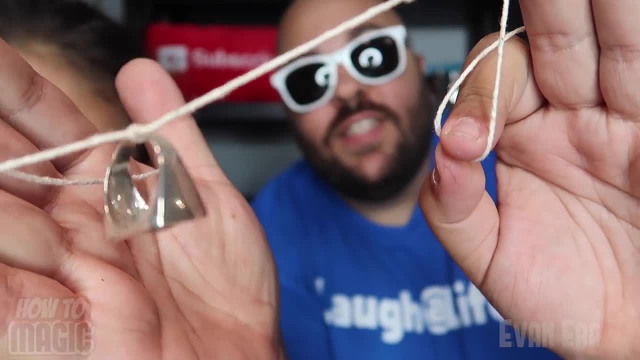 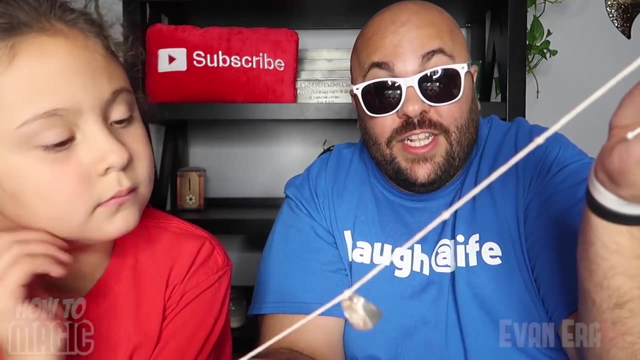 And the last one, The last knot over here with the ring on it. So once you have the ring tied on the string, this is how it's going to look at the very start, And you're going to do this before the trick starts, before you show it to anyone. 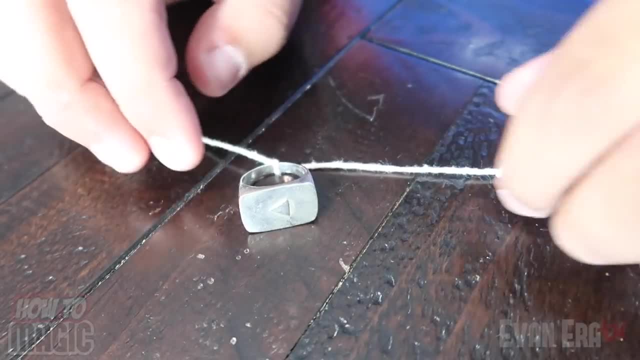 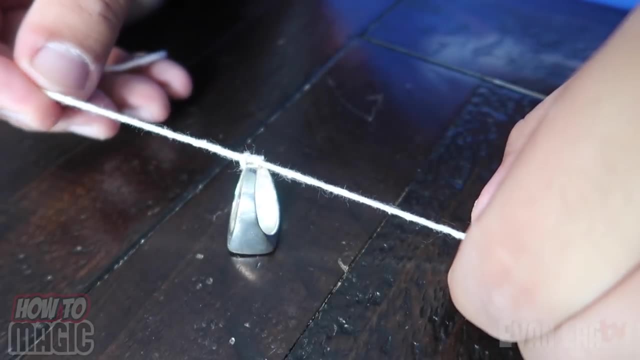 So you want a piece of string about a foot and a half to two feet long- You can also do this with rope- And you want to tie three knots about in the middle of the string: One there, one there And on the last one you're going to tie it around the ring. 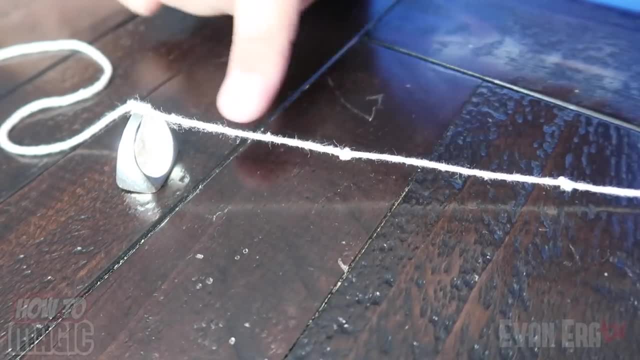 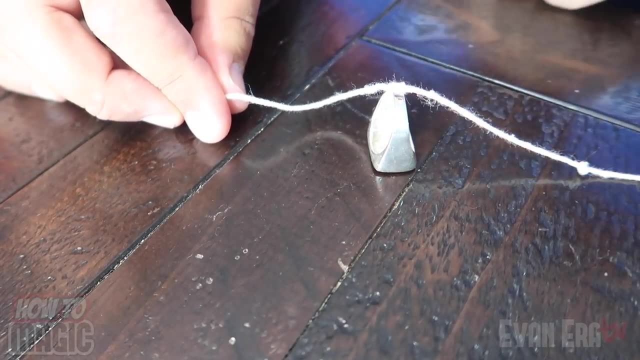 Now you want these to be equidistant from each other- just about two and a half, maybe three inches between each knot. Before the trick starts, you're going to come over here and you're going to tie a special type of knot on this side of the ring. 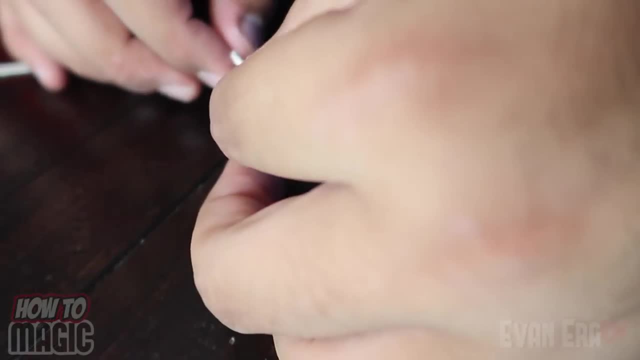 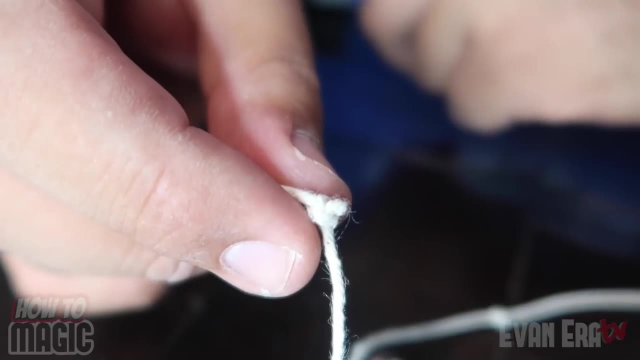 You've got your other two knots over here. You want to tie this knot over here on this side. You want to make sure that it's about the same distance between the other knots, about two and a half to three inches. It's going to tie what's known as a slip knot. 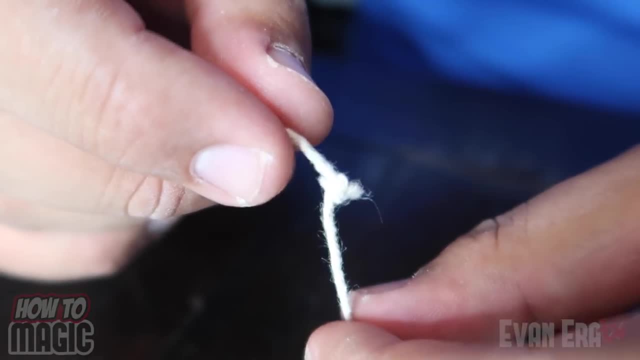 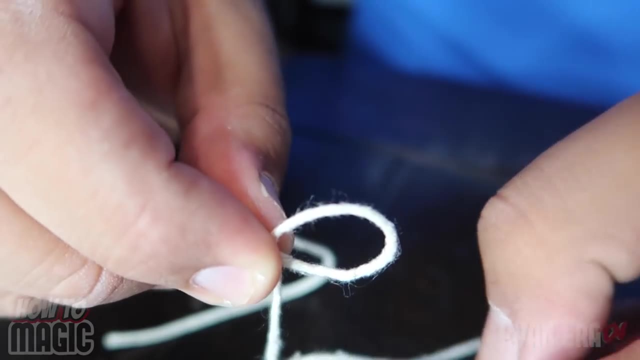 It looks very similar to a regular knot, but when you pull on it, the rope will straighten out and the knot will disappear. You simply wrap the rope around your finger and pinch the loop, Then create another loop, And that's going to go through the first loop you made. 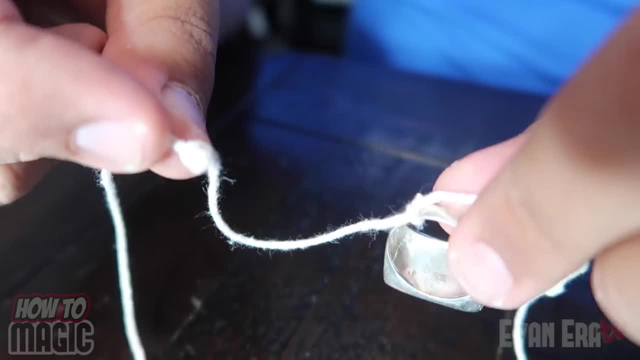 And that's going to go through the first loop you made. And that's going to go through the first loop you made. Then tighten it up. It may require some trial and error to get the knot in the right position. You want it to be equally spaced as the other knots. 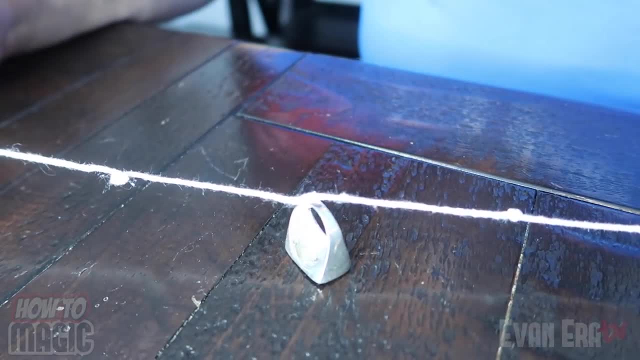 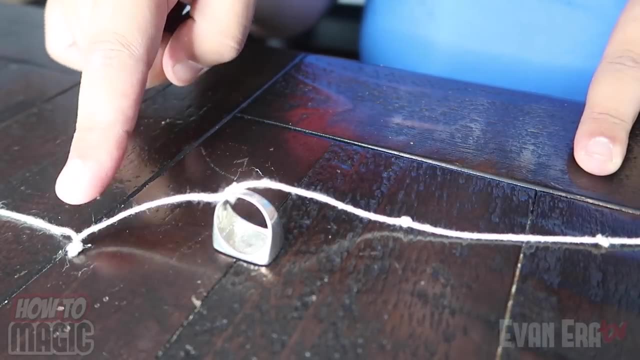 This one's a little bit too far out Right there And that looks pretty good as far as spacing now. Now we have four knots. We have the three real knots and the one with the ring here and we have the slip knot. 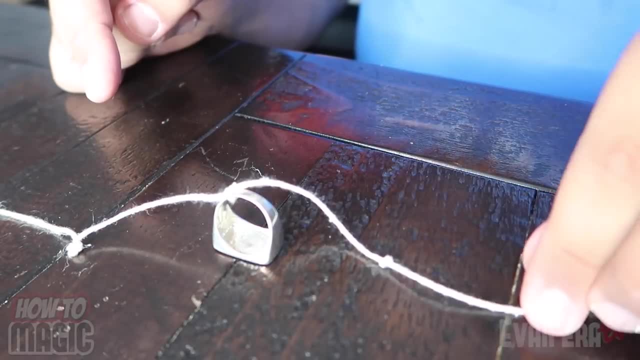 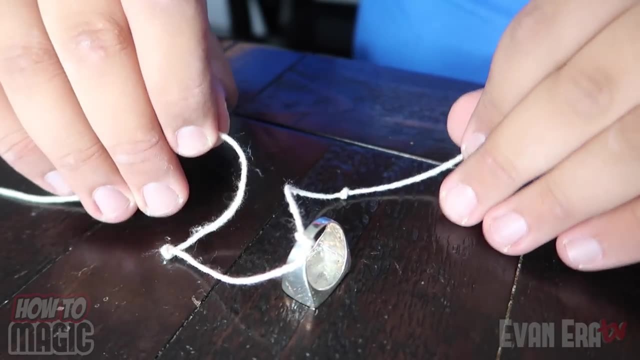 here. What we want to do is conceal this little knot right here in between our fingers, just like this, And pick the other side of the rope up right here. So now it appears as though we have the ring tied In the middle of the rope. 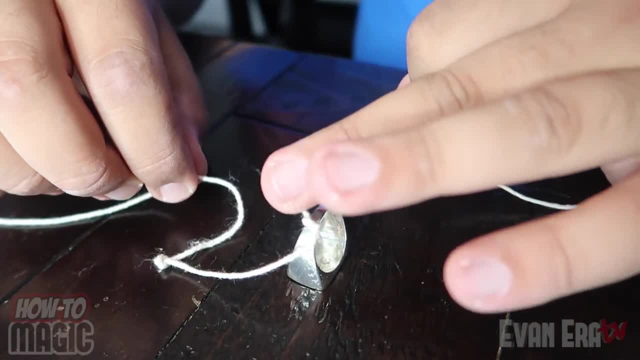 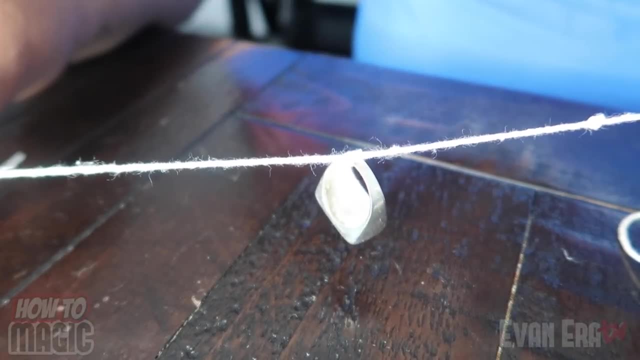 With two knots on either side. Now, to make it jump from this knot in the middle to this knot over here, all you have to do is pull the rope from either side. This knot will disappear, And you want to simultaneously pull two to three inches of rope out from these fingers. 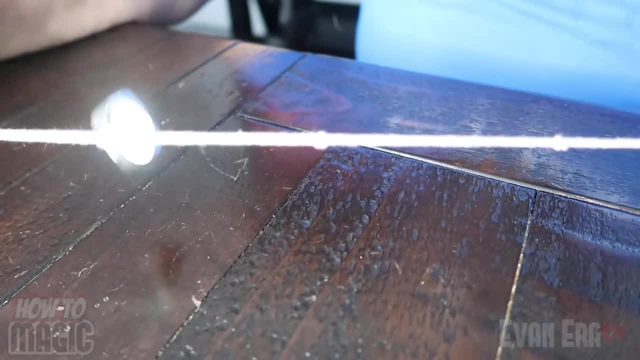 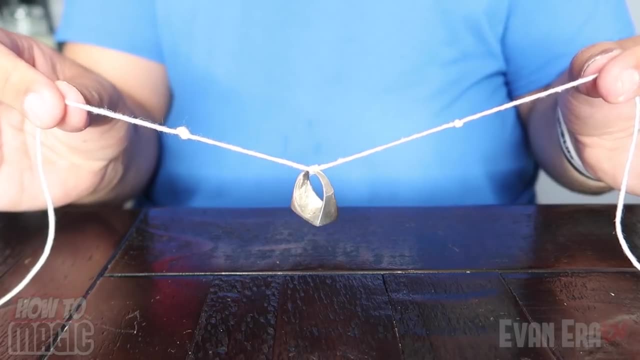 and expose this knot. So you're going to do that simultaneously and pop the string And it's going to look like the ring jumps from this middle knot all the way over to this one. So we've got the ring on the middle knot right there. 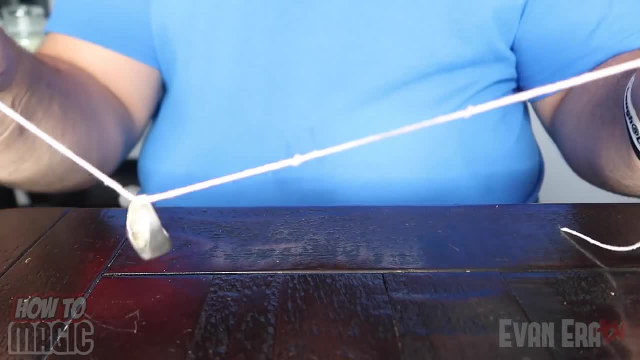 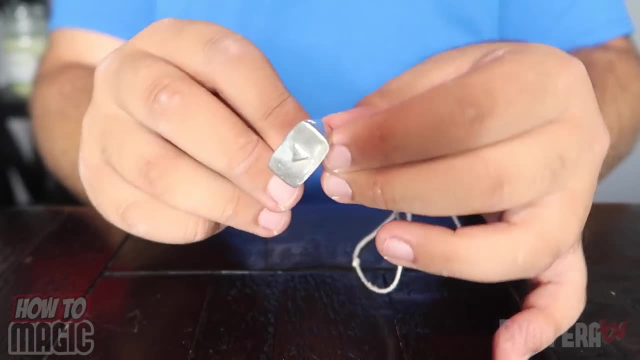 One, Two, Three And it jumps to the third knot. They can instantly inspect this and hand it out to the audience. That's the great thing about this is the ring really is tied on there. The other two knots are genuine as well, and you can use a borrowed ring. 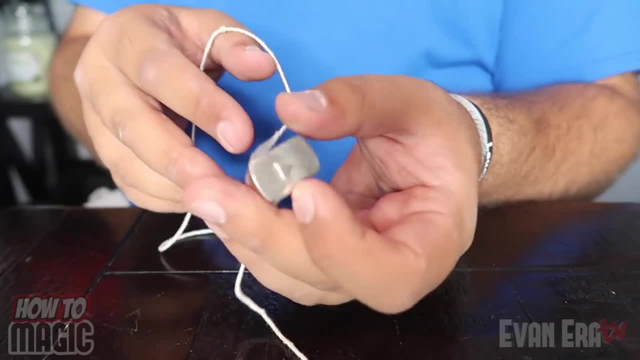 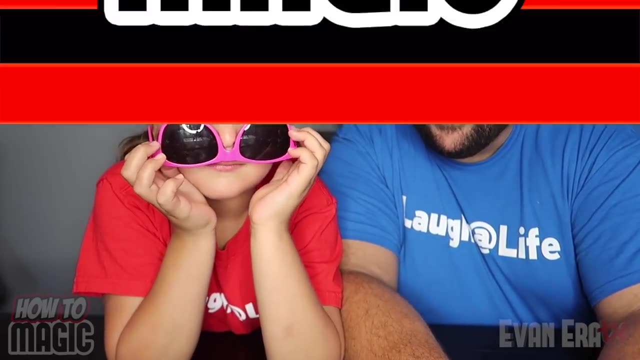 So you can borrow a ring from the audience, tie it on, tie your other knots and if you get really proficient at doing the slip knot, you can even do the setup in front of your audience. And that is how you do the magic ring and the string. 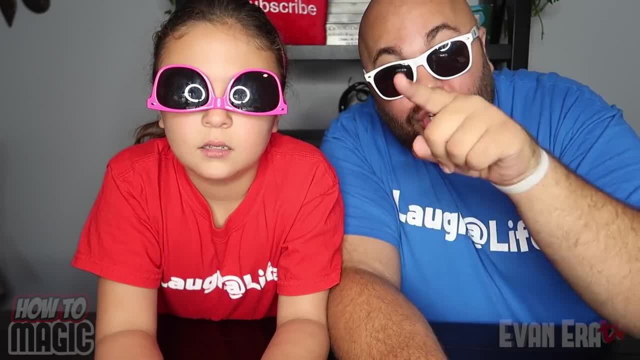 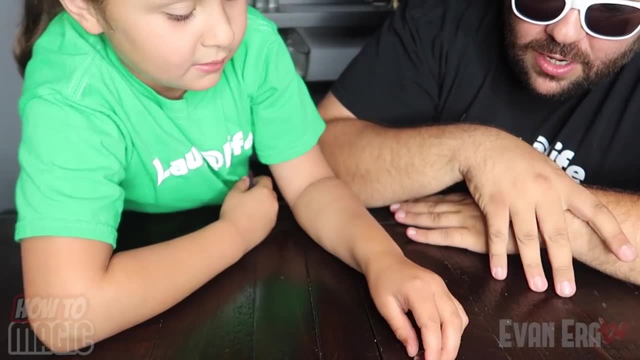 This one's a really easy, clean trick that you can do at home right now. Check it out. So I'm going to take this coin, put it down here on the table right there. Wait, can I inspect it? Yes, you might check it out. 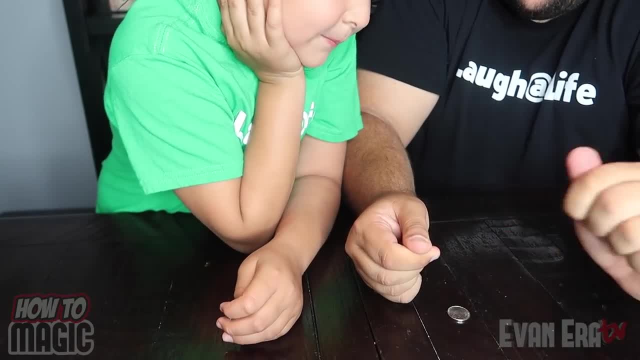 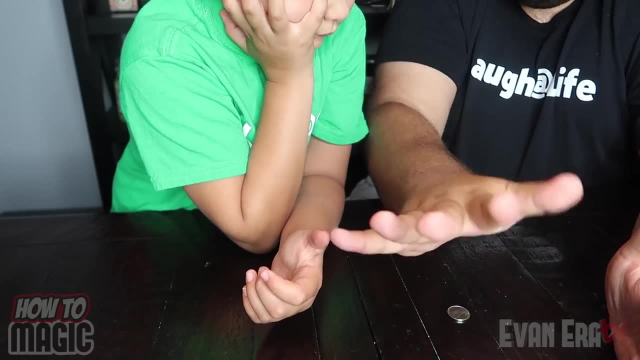 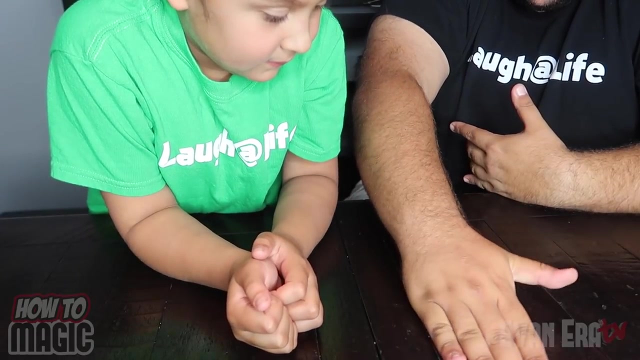 Seem normal. Okay, I'm going to sit that right there, okay. Now I'm going to take my hand and inspect the palm of my hand. It looks normal, right. Nothing tricky there. No fake hand Watch. I'm going to cover the coin with my hand. 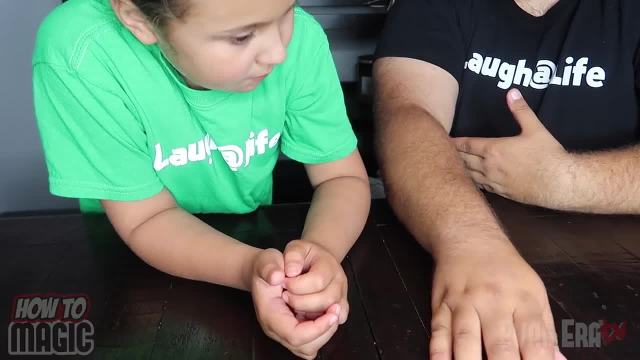 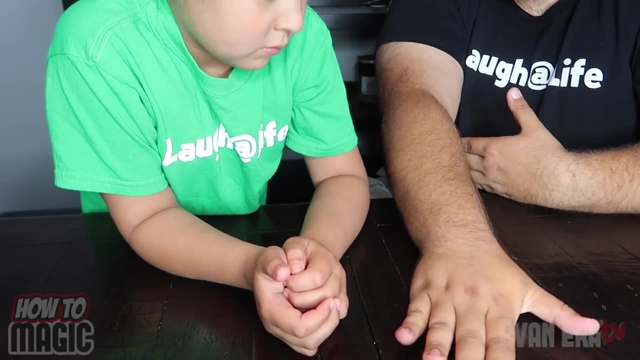 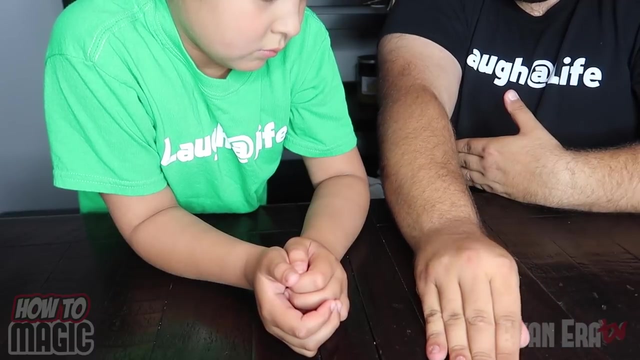 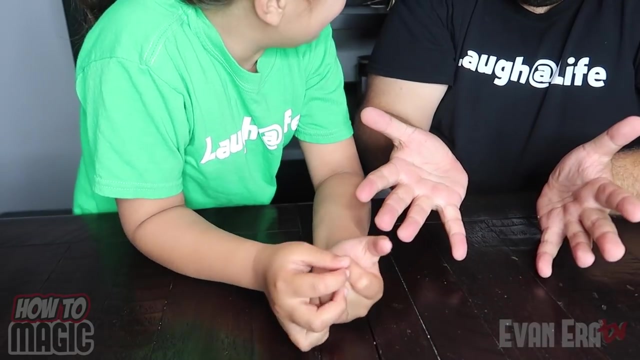 Now all I have to do is rub, Just rub the coin into the table. And if I just keep rubbing, How did it disappear? It went right through the tape. I think it's going to be on the floor. Oh my gosh. 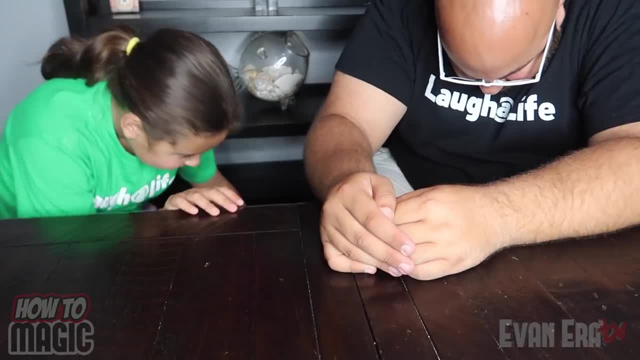 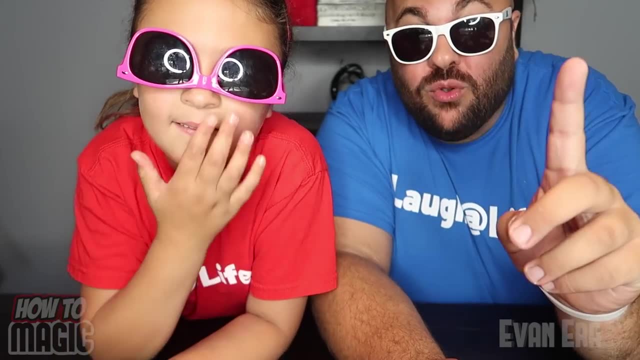 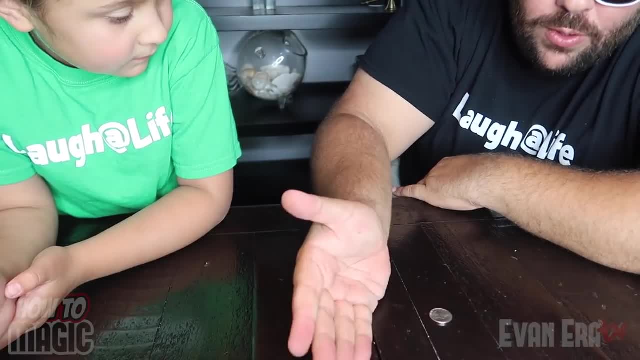 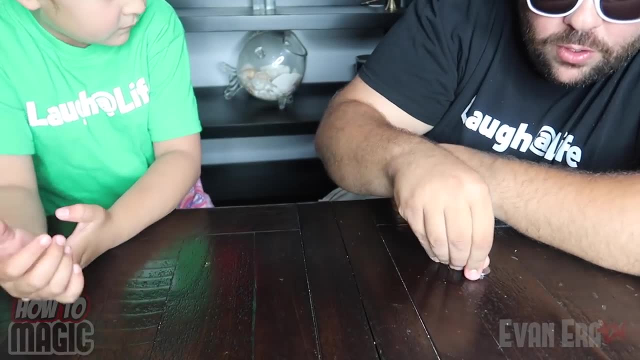 You're going to take the coin, sit it on the table and then you're going to cover it with your hand. Now, what they don't see is, during this motion, you're actually inching the coin back and letting it fall off the table, and that's hidden underneath your forearm. 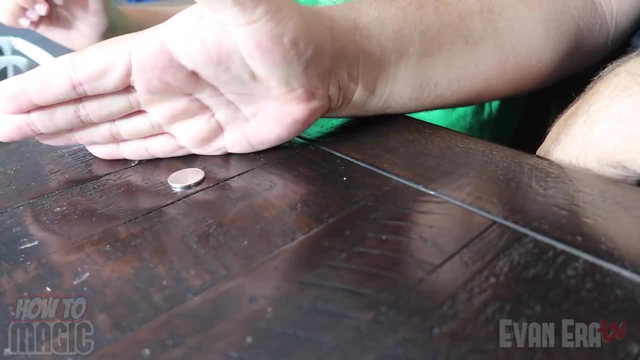 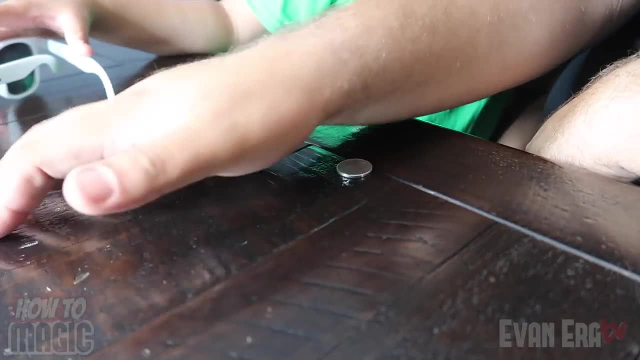 All right, so you're going to take the coin, sit it down on the table and then your hand is going to go right on top, like this. this now. what they don't see is when you do this motion, you're actually pushing the coin back with every move until you push it all the way off the table. now. 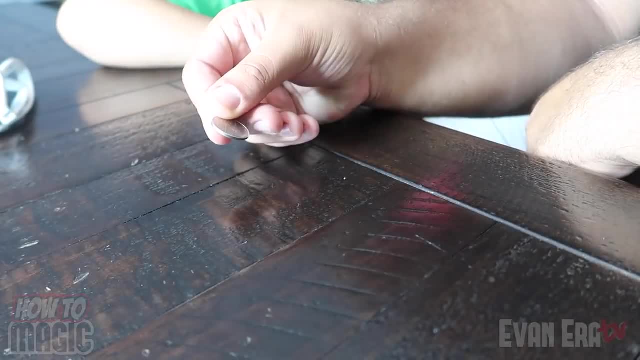 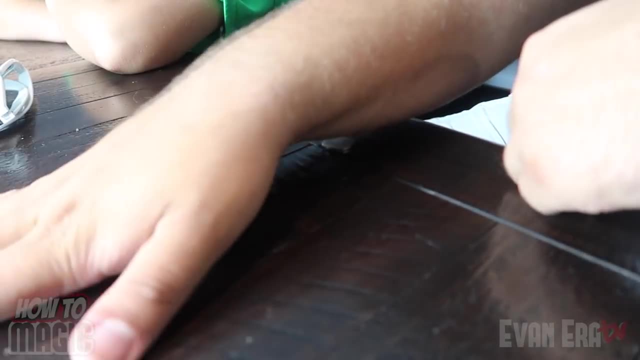 this happens under the cover of your forearm, so you can do this with pretty much any coin you want. to make sure it's pretty close to the edge of the table. forearm is going to cover the path of the coin right here, so as you inch it back, you're just gonna kick it off the table. this works best done over carpet. 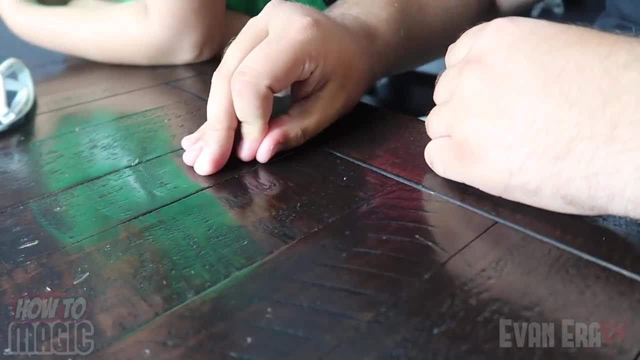 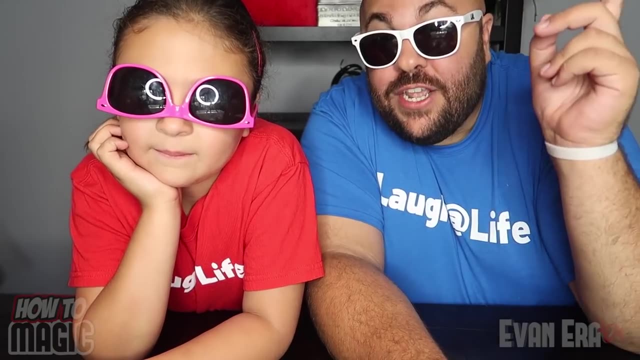 so the coin doesn't make much of a noise when it hits the floor. then you continue to rub and the coin disappears. super easy trick. try it out at home. and that is how you do the magic queen through the tape. okay, for this one you're gonna. 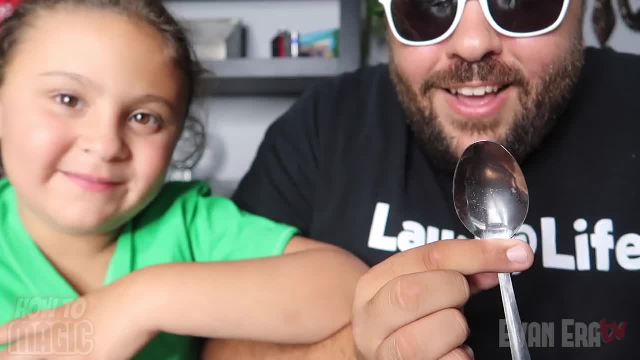 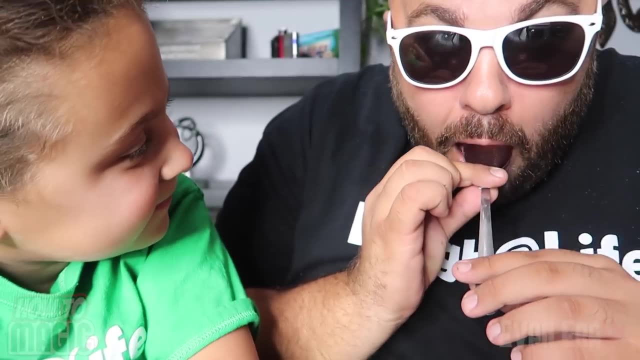 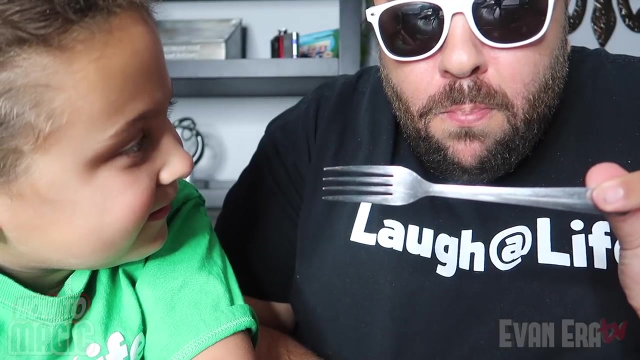 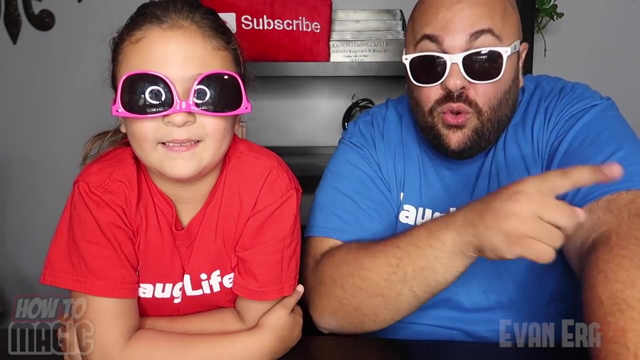 take a spoon and do something truly magical with it. take a look, okay, so I have a spoon here. check this out. I'm gonna take the spoon. watch watching. check this out. here's the explanation of the magic spoon into the fork trick. so this one's super easy. all you need is one of our magic bending spoons from the shop and 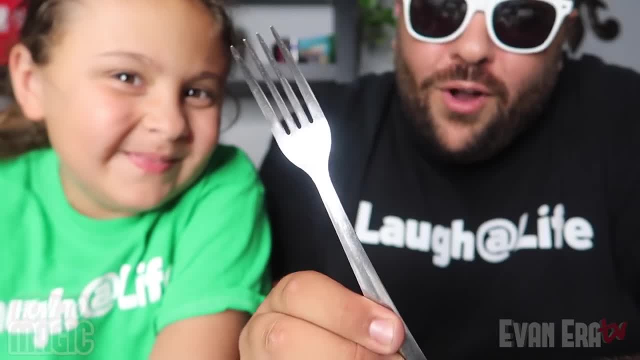 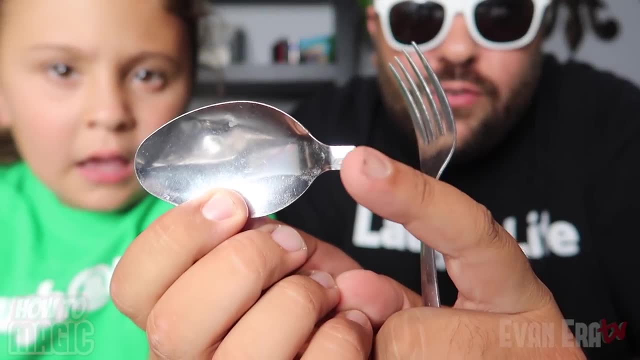 then you take this off, remove the top part sitting gonna take a fork- this is a regular kitchen fork- and you're gonna take the top half of our bending spoon. now you want to be careful because the way these are cut from the factory it can be a little sharp on the end. here you might get a parent to take some. 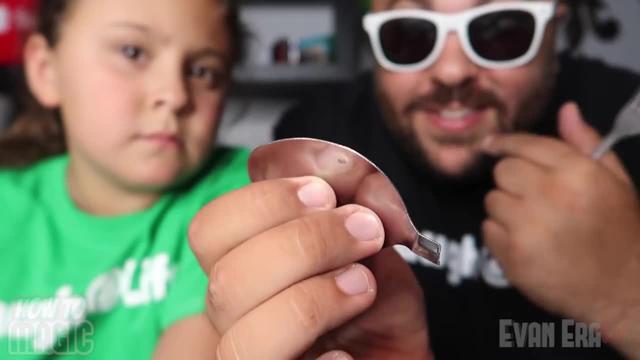 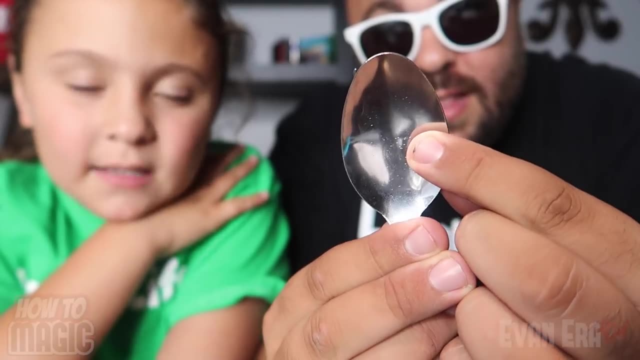 sandpaper and kind of sand it down so it's nice and smooth on the end. that doesn't cut the inside of your lip. so what you're gonna do is position the spoon right on top of the fork, just like this, line them up, just like that. 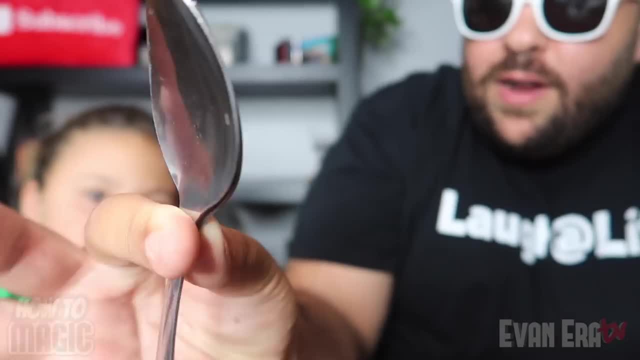 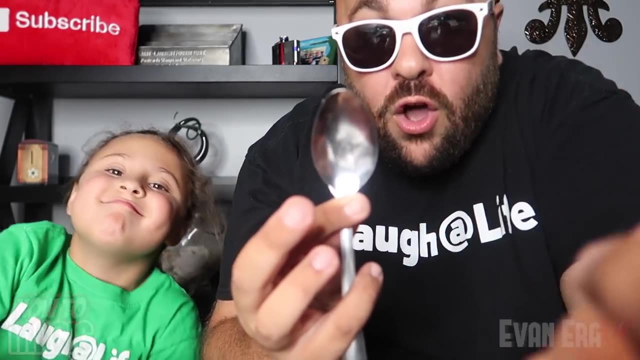 and you're gonna hold it right here with your fingers. now you're just holding that spoon piece right on top of the fork like that, and it's concealing it behind it. now this would be visible to an audience on either side of you. so you want to perform this for somebody straight on, so you take the spoon come. 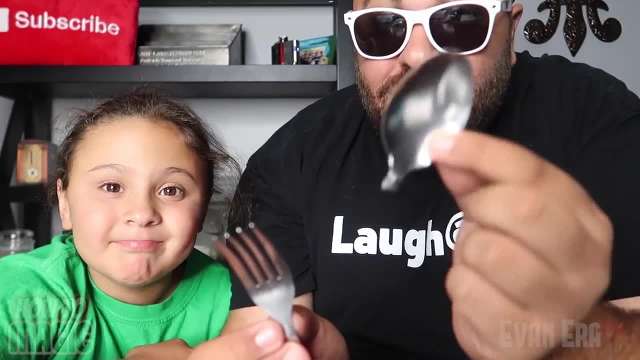 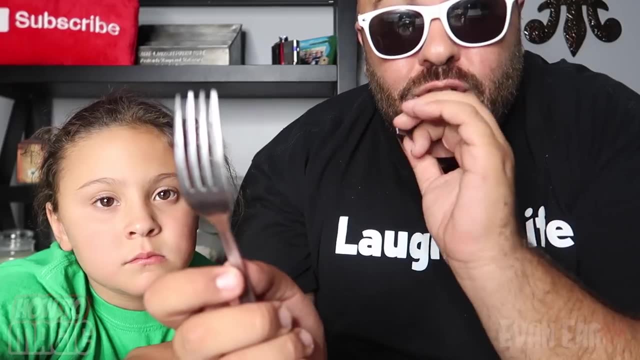 up to your mouth. the spoon goes inside with the fork and you just leave this part of the spoon in your mouth. now you can't really talk at this point, but you can immediately hand the fork to them. hopefully all of their focus will be here, and then you can spit the spoon out and ditch it into your pocket. 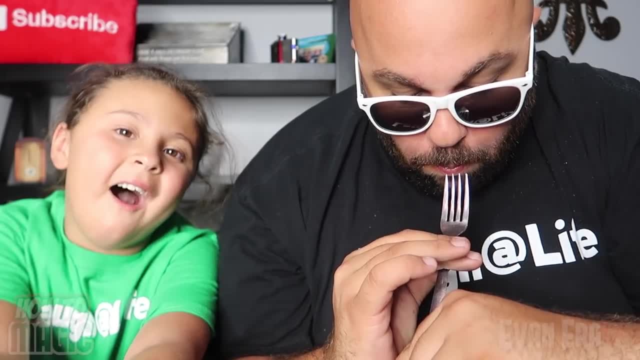 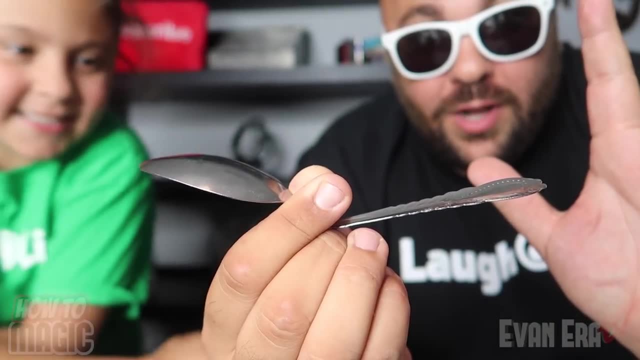 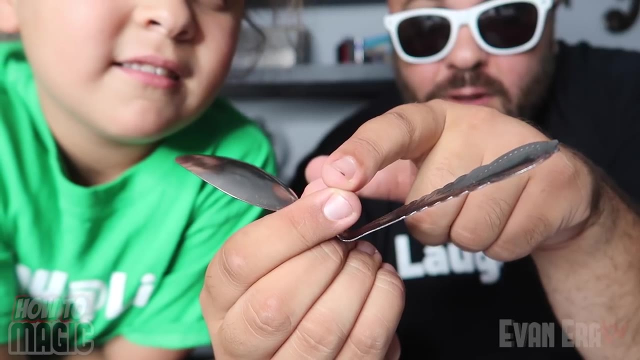 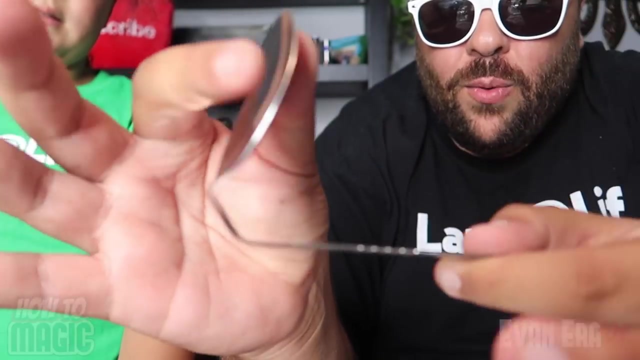 Oh, So this is our bending spoon that we sell in the shop. super cool trick. Look at that. Look at this happen And it will keep bending until it bends all the way in half Real metal. And that is how you do the magic spoon and fork trick. 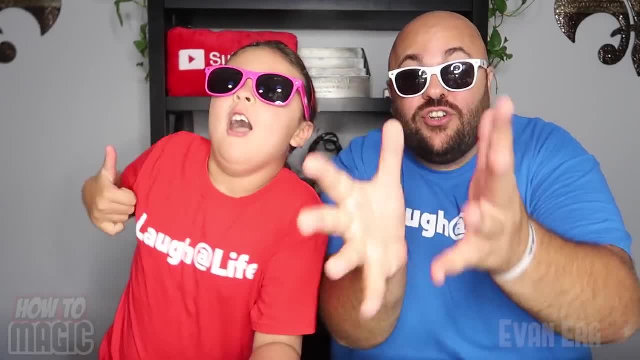 All right, guys. if you liked all those fun magic tricks, give this video a thumbs up and be sure to head over to the Evanera TV shop. That's howtomagicshopcom. There's a link in the description. You can also go to evaneraTVcom. 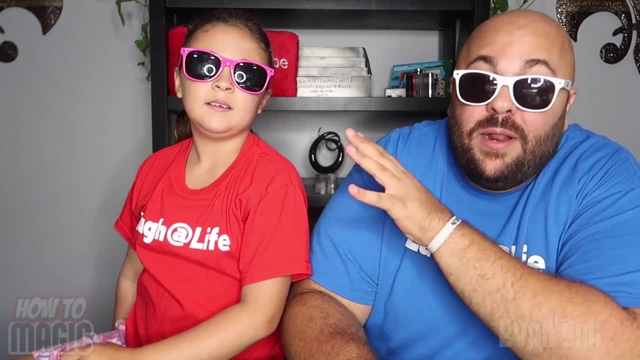 They both take you to the same site. Head over to the shop and pick out a cool Laugh at Life tee. We have them in a bunch of fun summer colors available for kids, ladies and men. We also have our Laugh at Life shades for sale. 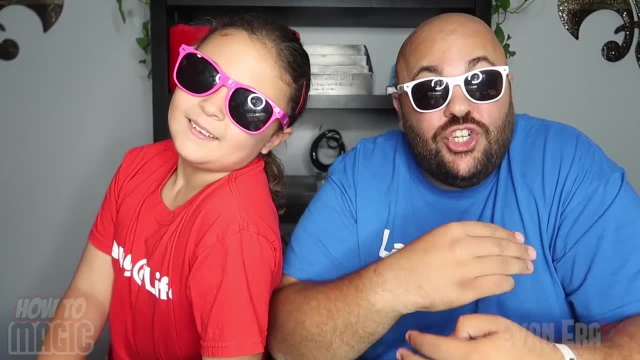 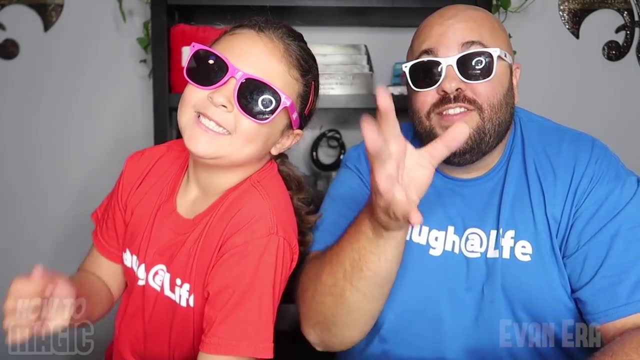 You can get a Laugh at Life wristband and we have a bunch of cool magic tricks. We ship everything international. We have international shipping available on all items, all our magic tricks, and we have a lot of new products coming soon. Be sure to keep checking back on the site daily. 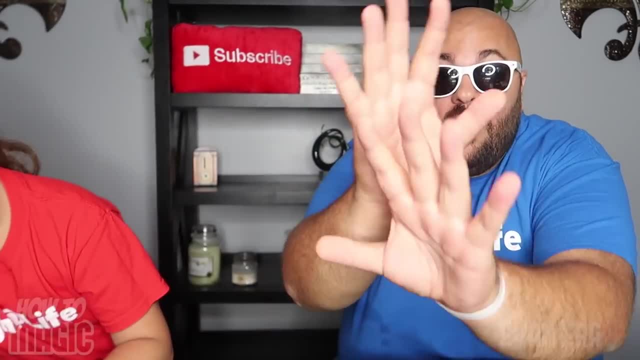 You'll be the first to get your hands on the new products. Guys, if you have a Facebook account, go follow me on Facebook. right here, It's Evanera TV. I'm posting a lot of cool videos there- almost a video every single day. 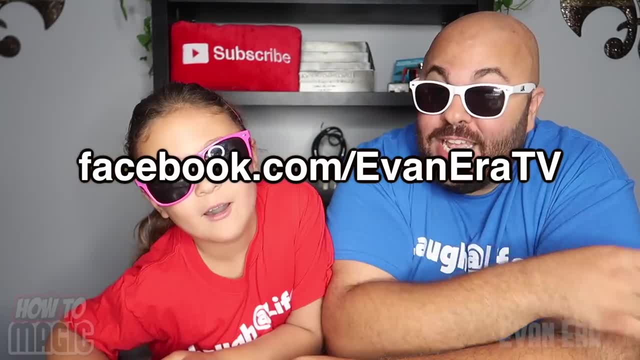 And the Facebook page is blowing up, so be one of the first people to like the page and give it a follow. Yes, The link for that is in the description. All right, guys, if you don't know about our second channel on YouTube, that is Evanera. 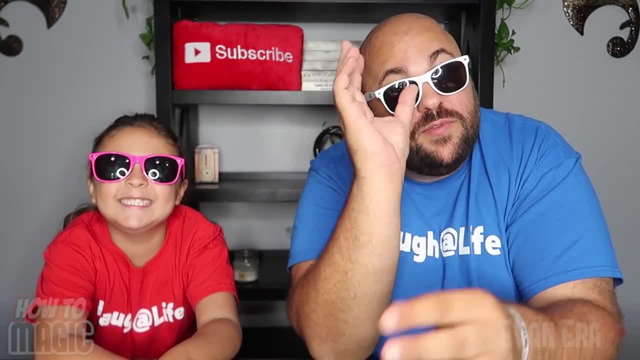 Vlogs. We post a lot of fun videos there as well, So if you haven't yet, go subscribe to that channel and watch a video. All right, guys, it is giveaway time. I am giving away five magic bending spoons from the Evanera TV shop. 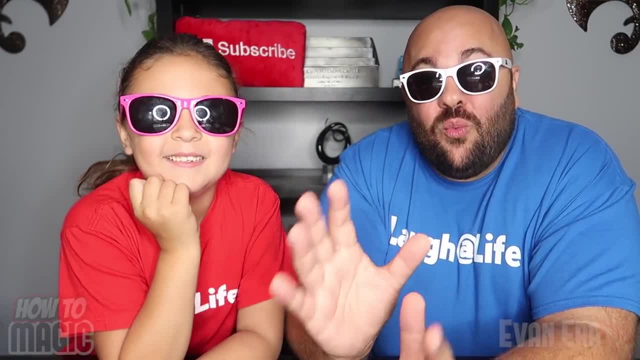 To five lucky winners. You can leave as many comments in the comments section below. All you have to do to be eligible to win the giveaway is give this video a thumbs up, leave a comment in the comments section below and be subscribed to this channel. 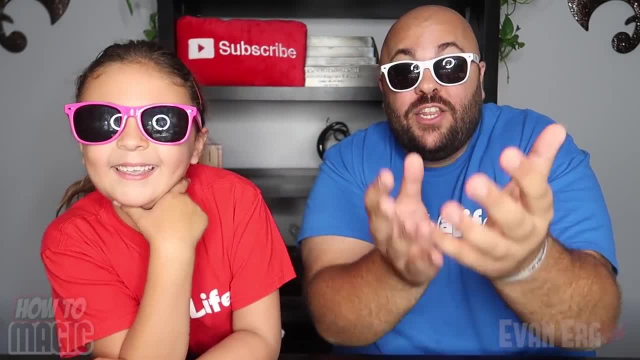 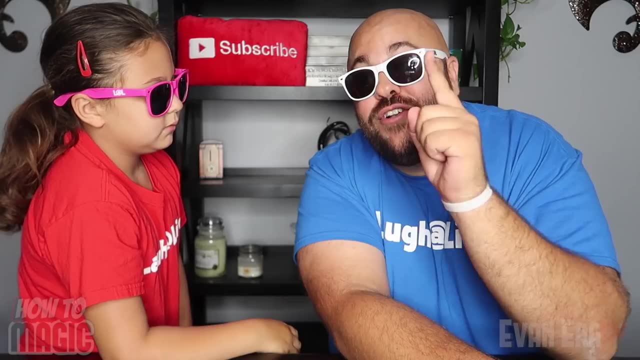 Today's keyword is magic, So leave a funny random comment using magic. in the comments section below, You can leave as many comments as you want- unlimited comments, In fact. the more comments you leave, the better your chances of winning the giveaway.